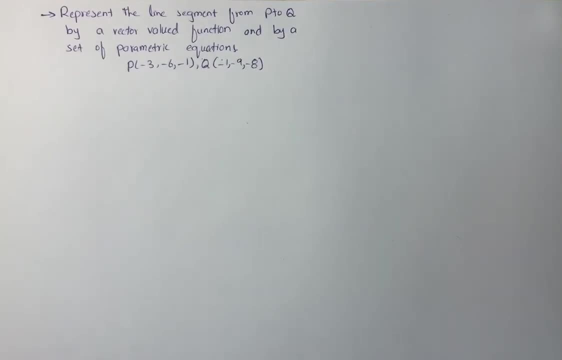 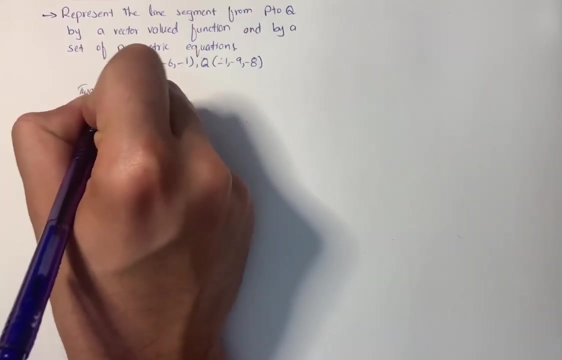 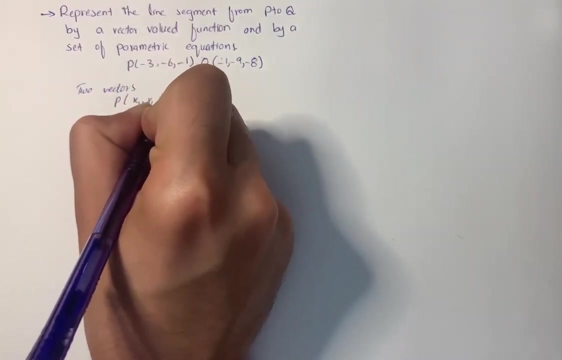 so the question says: represent the line segment from p to q by a vector valued function and by a set of parametric equations. so p into minus 3 minus 6, minus 1 and q into minus 1 minus 9 and minus 7. so two vectors are here, two vectors, that is, p into x 1, y 1, z 1 and q into x 2, y 2. 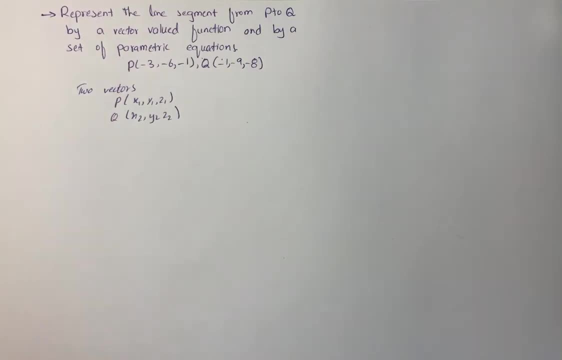 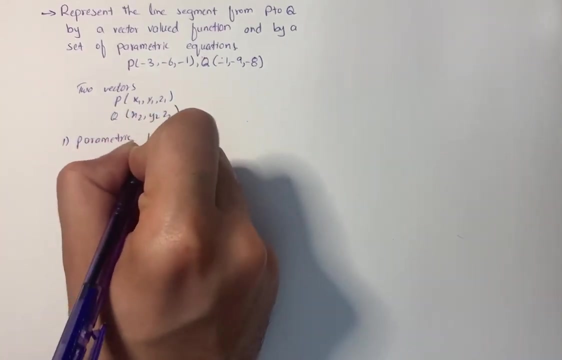 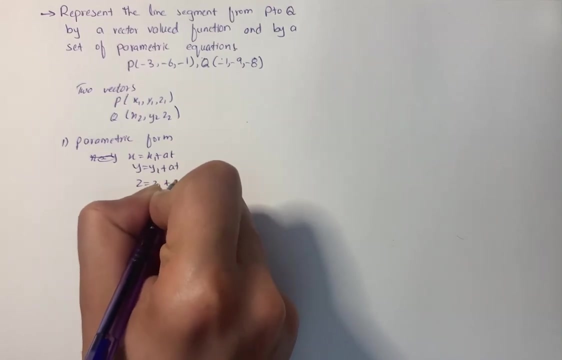 and z 2. now the line segment from p to q parametric form is. parametric form is: x is equal to, x is equal to x 1 plus 80, y is equal to y 1 plus 80 and z is equal to c 1 plus 80, where a is equal to. 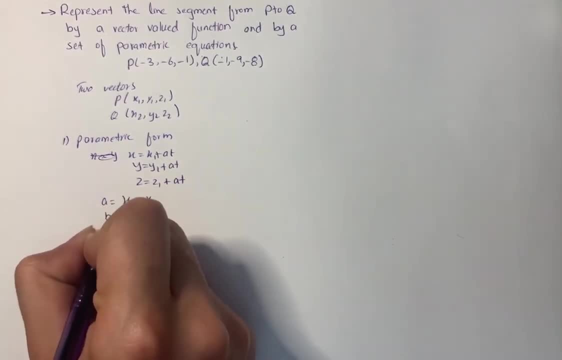 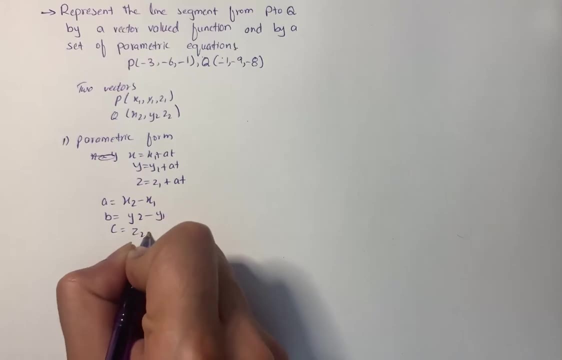 x 2 minus x 1. b is equal to y 2 minus y 1 and c is equal to z 2 minus z 1. now the vector valued form is. vector valued form is: r equals to x, y z. so for the second step, 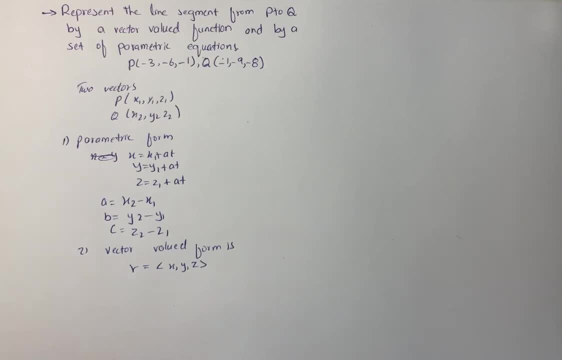 the given vector. first we will evaluate a, b and c. evaluate a, b and c, so we have p. q equals to x 2 minus x 1, into y 2 minus y 1, into z 2 minus z 1. on putting values, it will become: 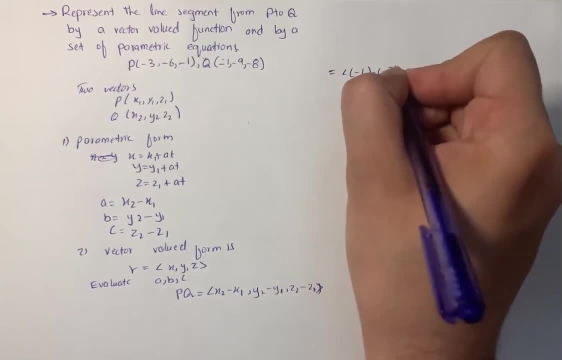 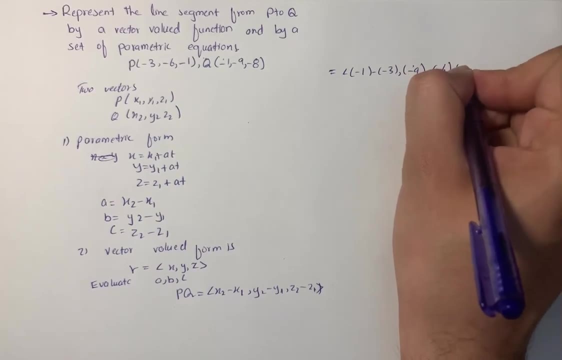 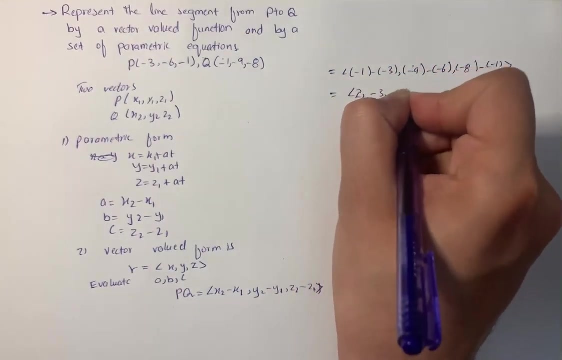 minus 1, minus into minus 3, into minus 9, minus into minus 6, into minus 8 and then minus 1. that's what we have over here, and on solving it would give us 2 minus 3 and minus 7.. now the parametric form is: